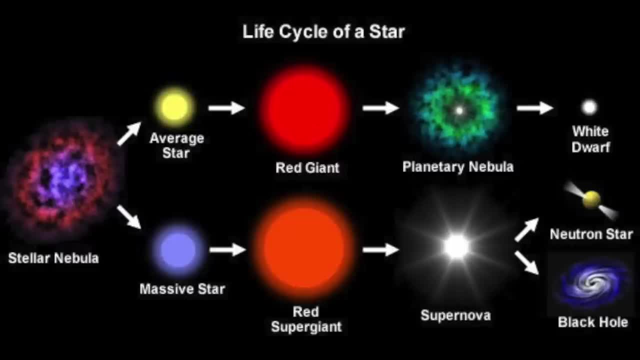 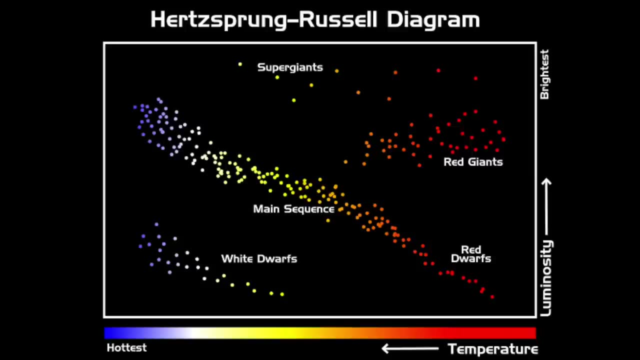 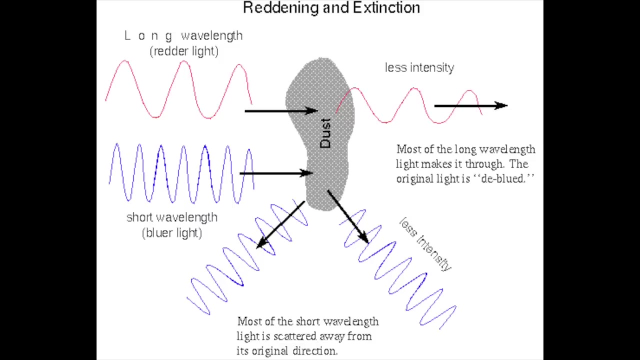 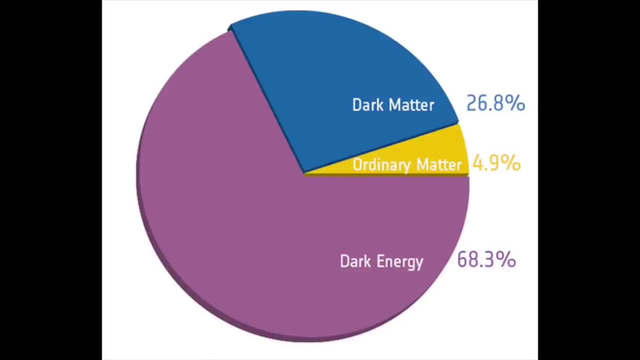 physics, maths and computer science, plus a couple of specific astro courses covering stellar evolution like the Hurt-Sprung-Russell diagram, exoplanets, galaxy structure, interstellar dust, Hubble's law, dark matter and dark energy. This shouldn't be too hard if you've done any reading or independent. 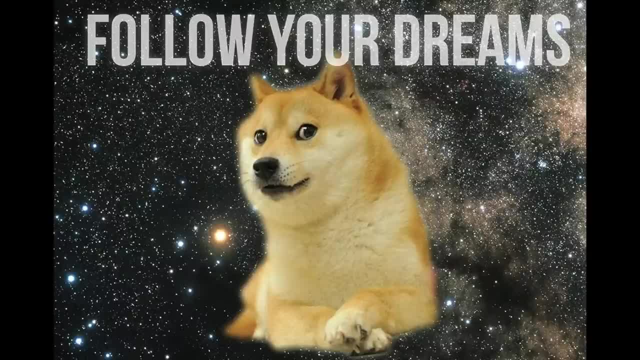 research on the subject. Even more so than physics, astronomy attracts people who are really passionate about the subject from a point of interest rather than job marketability. So you probably know a bit about these subjects already. Moving into higher years, you will cover astronomical imaging. 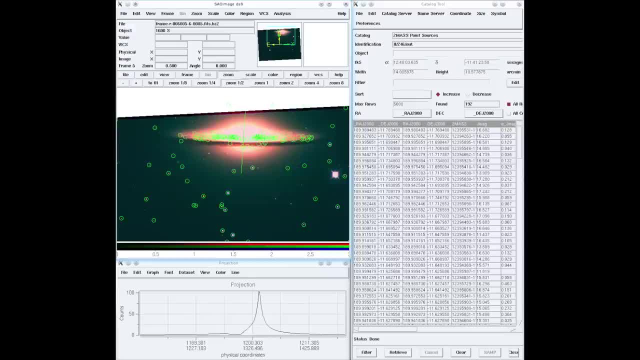 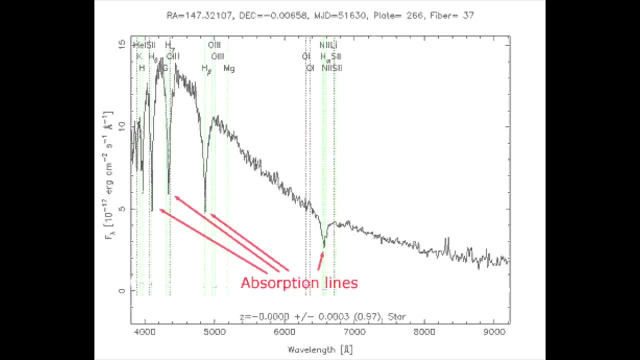 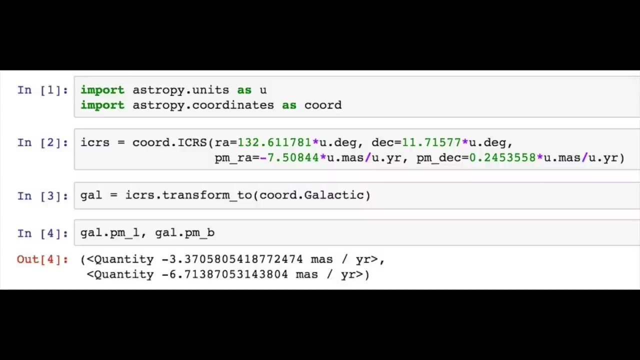 usually through a hands-on course where you use computer programs such as DS9, MATLAB and Python to process images, apply filters, perform astrometry, which is measuring positions of stars and spectroscopy. This is where you will really start to see the benefit of taking computer science courses. 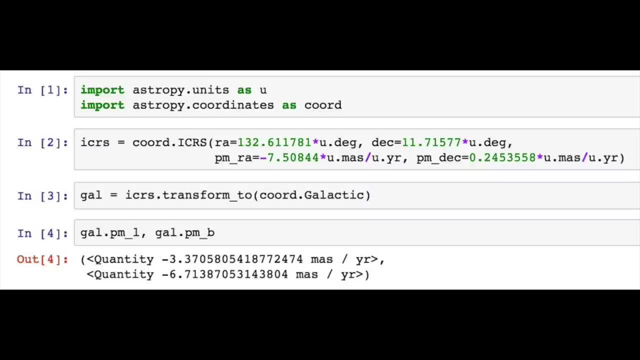 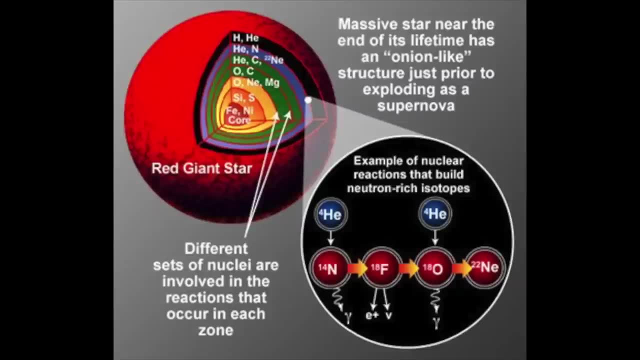 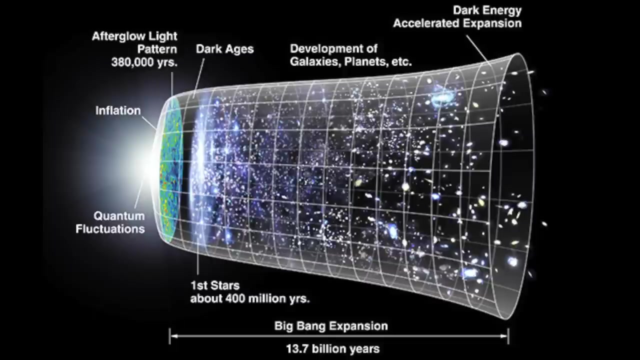 Astronomy involves a lot of data and it's not very useful to you unless you know how to manipulate it. Additional astro courses might go further in depth about topics like nucleosynthesis, which is how elements are created, or solar system astronomy, cosmology, which covers the big bang and origin of the universe. 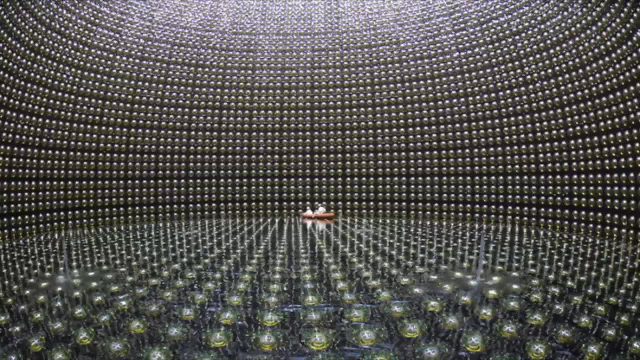 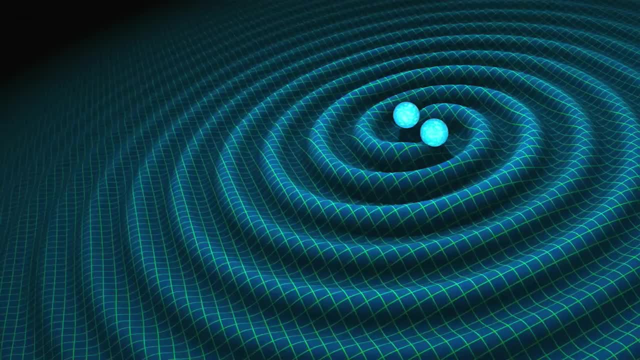 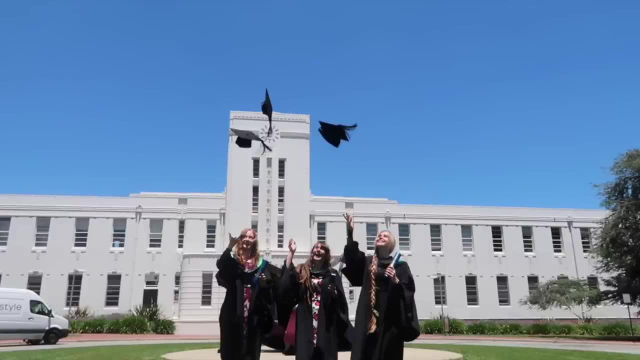 astroparticle physics, neutrino astronomy, planet searching or even gravitational waves. How much you get to do depends on which uni you're at. Where I did undergrad, there were only a couple of higher level astro courses And, truth be told, that even though I took some astro, 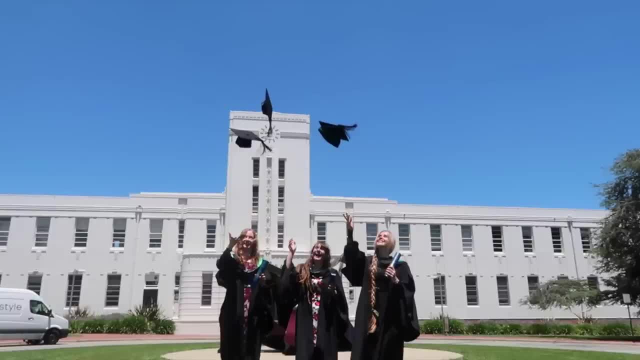 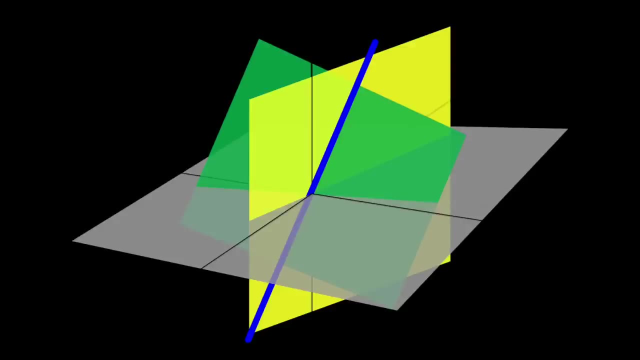 I ended up majoring in physics and math instead, because those were the subjects that were really the grunt work behind the astro topics and I was more interested in them. You will not be able to do astronomy without some solid knowledge also in linear algebra. 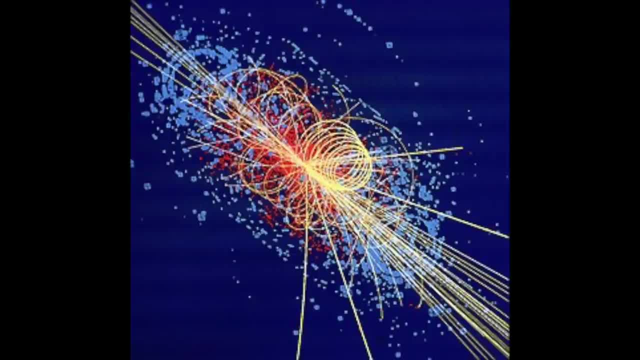 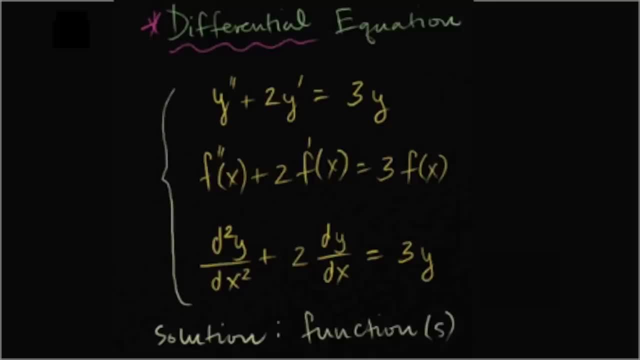 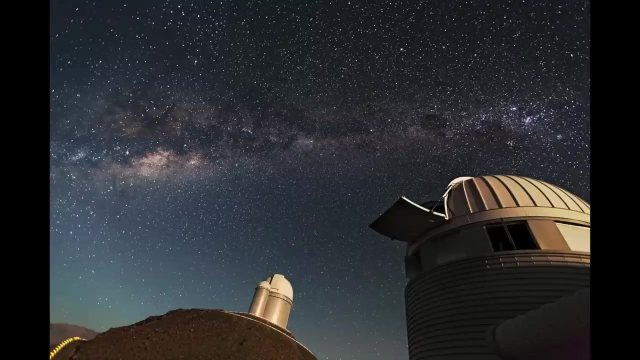 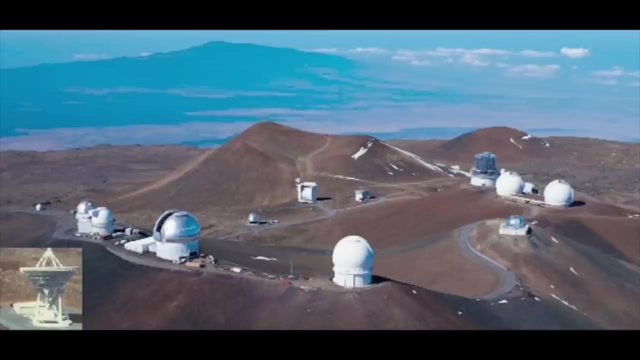 classical mechanics, nuclear physics, particle physics, orbital dynamics and differential equations And, unlike some astro ideas, these topics are harder to teach yourself as sort of a side hobby. There are plenty of cool opportunities for the astro major. A big one is working in research and working in any of the amazing observatories all over the world. 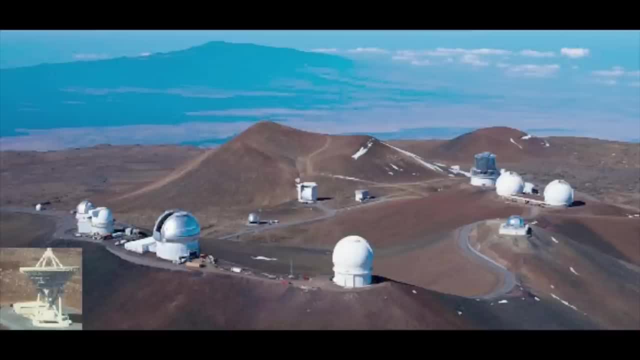 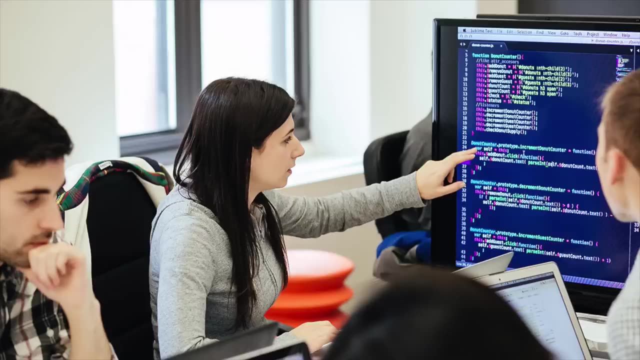 Either as a scientist or a technical staff or an outreach coordinator. Since you'll have math, physics and comp science skills as well, you can also work for companies that need someone technically minded. You could develop scientific software or electronics, and 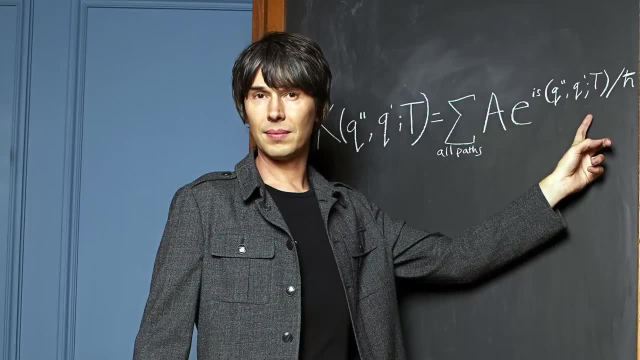 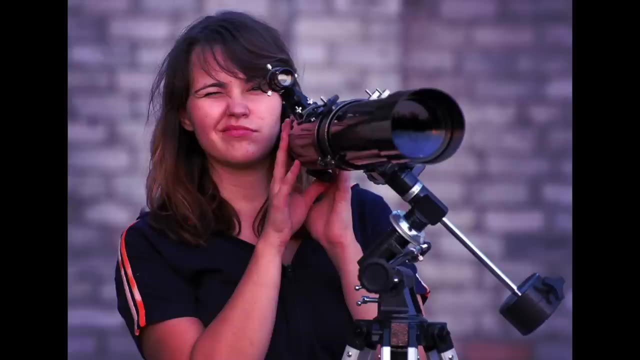 optics systems. You could work in science, communication, management or as a patent agent like Einstein. One thing you won't be doing much of whilst studying astronomy is looking through a telescope. You might do that for fun with your friends, but professional astronomy uses huge telescopes. that 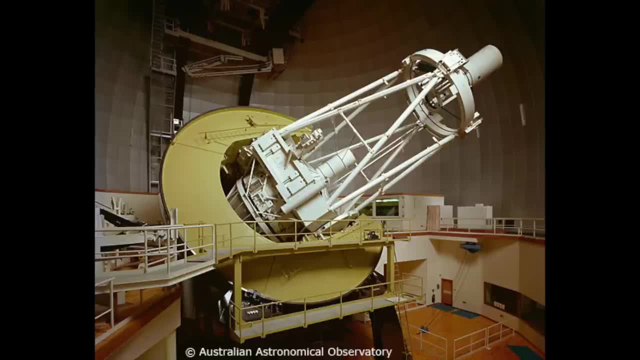 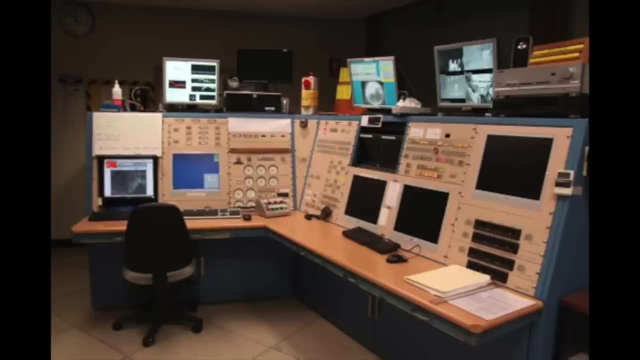 record data straight onto ccd cameras And then you are sent the data to process. You could be a successful astronomer without even using a telescope. If you do want to use an instrument for your research, you can use the telescope for yourself. then get prepared for some field trips, pulling all-nighters to 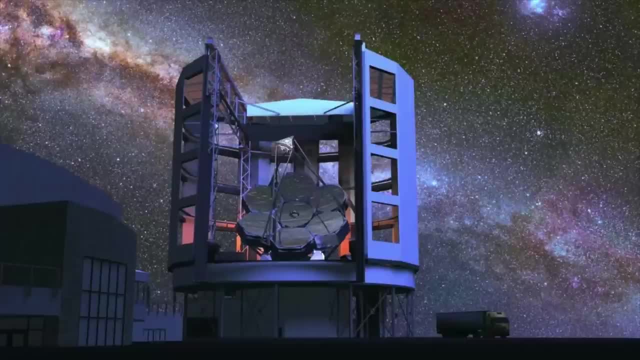 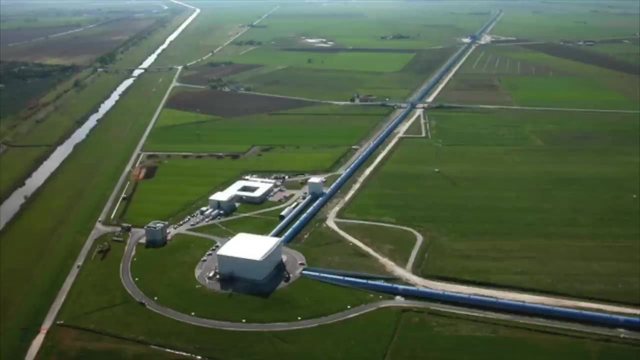 gather data. It's an exciting time in the astronomy community. There are some massive new global projects going ahead, such as the giant Magellan telescope being built in Chile, ready in 2023.. Then there's the James Webb space telescope being launched in 2019 and the new era of gravitational wave astronomy. So in 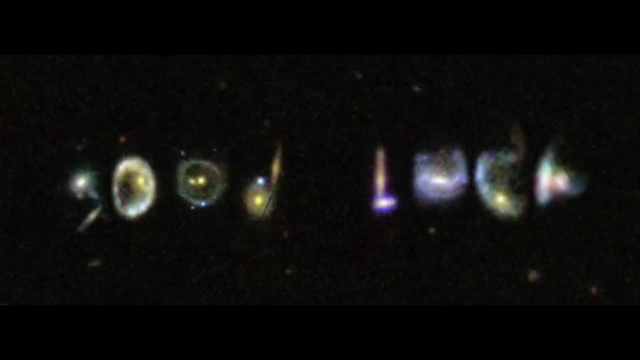 fact, it's a great time to get involved, as there will be a lot of data needing curious people to use it and find out new truths about the universe. So good luck.